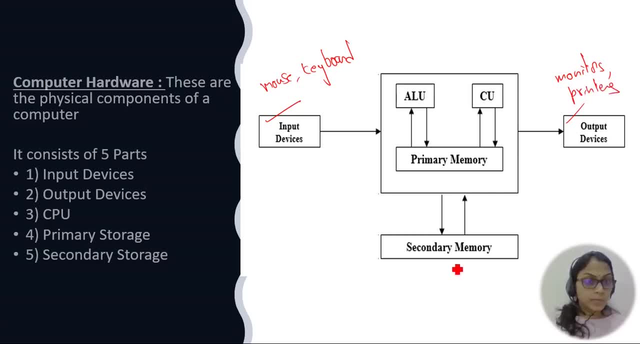 So these are all the output Devices. and coming to the secondary memory, Secondary memory is nothing but your hard disk- Okay, hard disk- and your pen drives. So, whatever the external storages or all come under the secondary memory. and what is the primary memory? 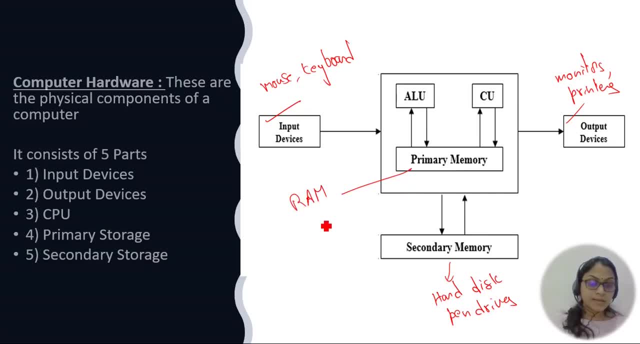 Primary memory is nothing but the RAM, Random access memory which is present inside your system. It is the fastest storage device and it stores, It takes The data from secondary memory and it plays whatever the executable files are. that opened files from the secondary memory. 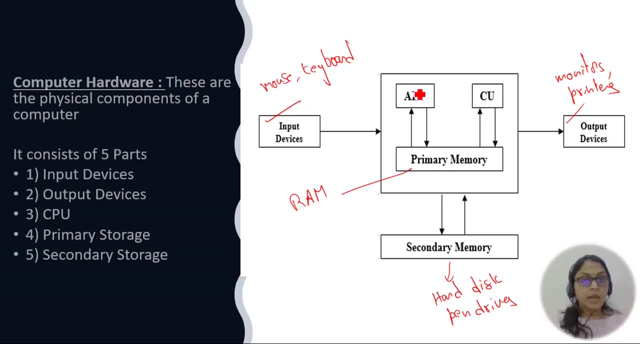 So that files will store on the primary memory. and ALU, ALU It's performs all arithmetic and logical operations and control unit is going to control the all the operations. So from where we have to get the data, where you have to send the data, everything the hardware control signals will be sent by this, operated by this control unit. 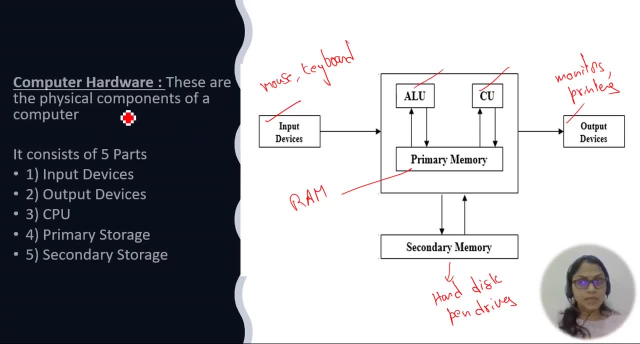 So the output is a one. Okay, so a computer hardware as a physical component of a computer. First thing is it is a physical component of a computer. That means you can touch and feel all the hardware components, or you are able to touch and you can feel it. 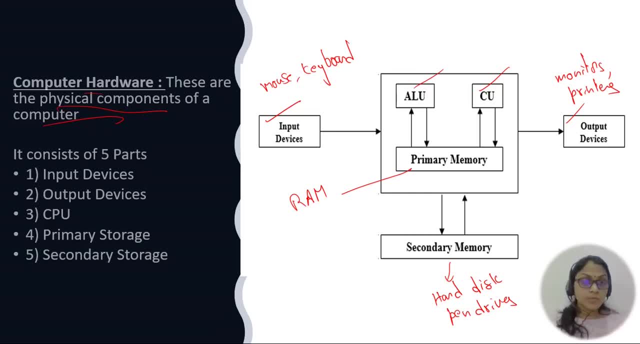 Okay, Those paths you call it as a hardware paths, So that's where we call those as a physical component. So mainly the computer hardware can consist of input devices, output devices, CPU, primary memory and secondary storage. So just remember this, It'll be faster. 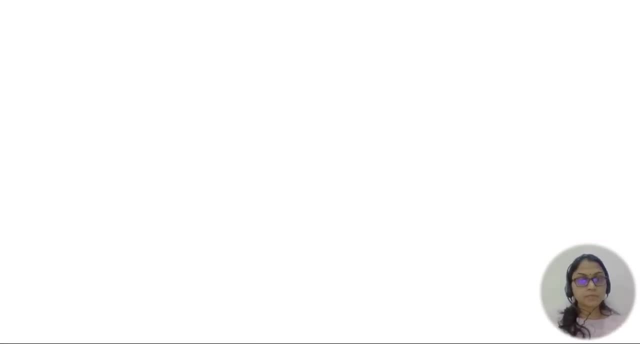 this block diagram. uh, now let's see what are the input devices in detail. so these are used to enter data. so these input devices are helpful, uh, helpful, in entering the data. so, with the help of the keyboard, you are typing the data. with the help of the mouse, you are navigating to one screen, to. 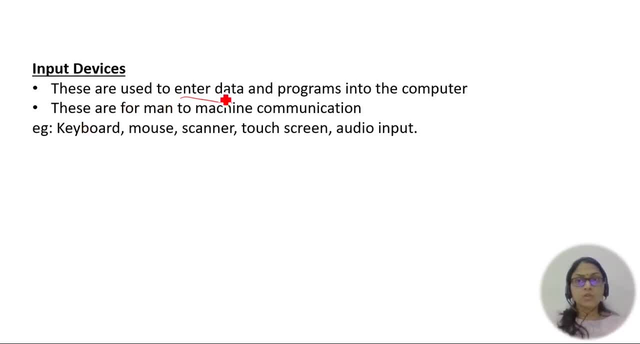 another screen and you can navigate to anything. okay, so these are used to enter data and programs into the computer and these are of man to machine communication. so we are the man, so we are the people, and to machine. so if you want to communicate this user to the machine, uh, this input device. 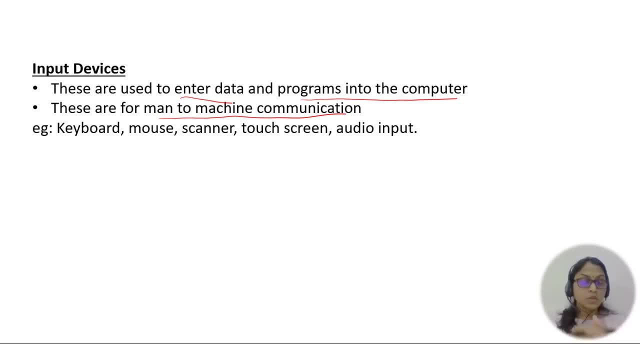 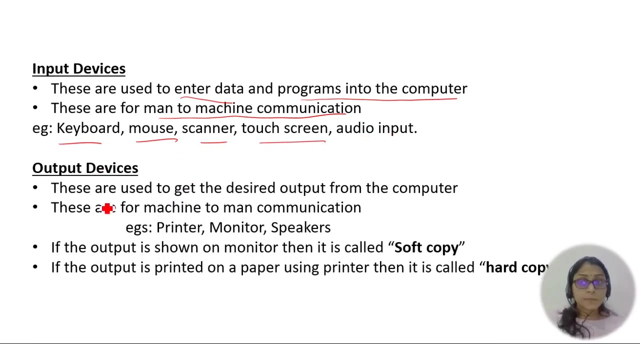 acts as an interface. okay, so these are used. these input, all these input devices, the keyboards, mouse- are used to uh for communication from man to machine. example, keyboard mouse scanners, touch screens and audio inputs, or all comes under the input devices. okay, you got an idea about the input devices. then what about the output devices? these are used to get the desired output. 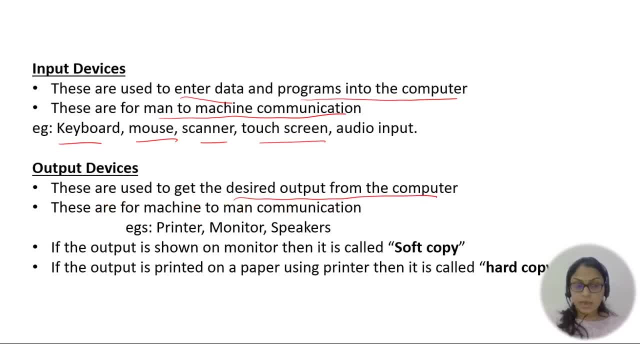 from the computer. so whatever the user has given, so it cpu is performing the operation and the result will be displayed, so that that is going to displayed on the output devices. so these output devices are used to get the desired output from the computer, from the computer computer. these are for machine to man communication. see the difference here. 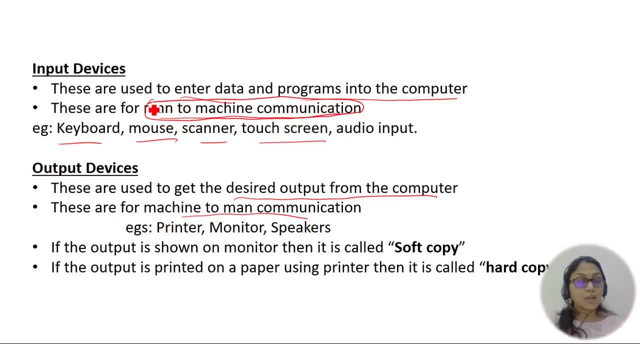 input devices, or you call it as a man to machine communication, whereas output devices are called as machine to man communication. so from machine we are receiving the data with the help of output devices, the different output devices or printers, monitors, speakers, if the output is shown on monitor, suppose if you are able to see the output on the screen. 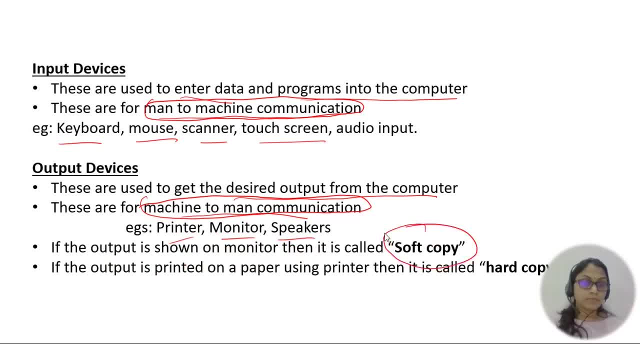 then you call it as a soft copy. some people may get means the basic uh, the starting uh using the system. if those people will get a confusion of what is a soft copy and what is a hard copy, soft copy is nothing but the output that is shown on the monitor, if you are able to see. 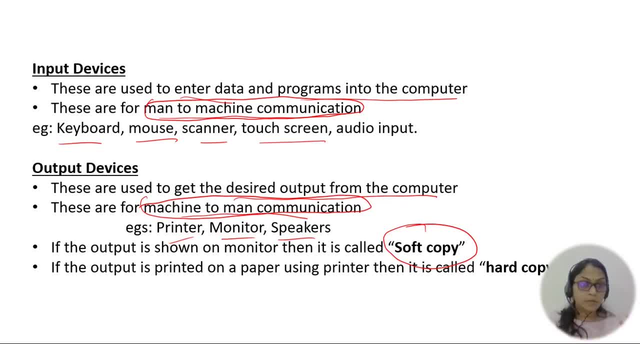 everything on the monitor that you call it as a soft copy. okay, you can't touch and feel it. okay, you are able to see that. that's it and the. if the output is printed on paper using printer, then you call it as a hard copy. hard copy means you can uh, see your data on the 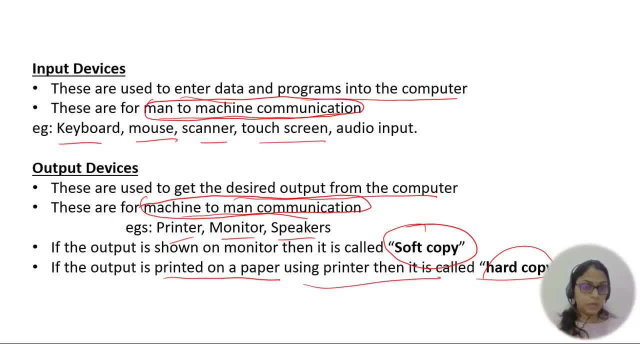 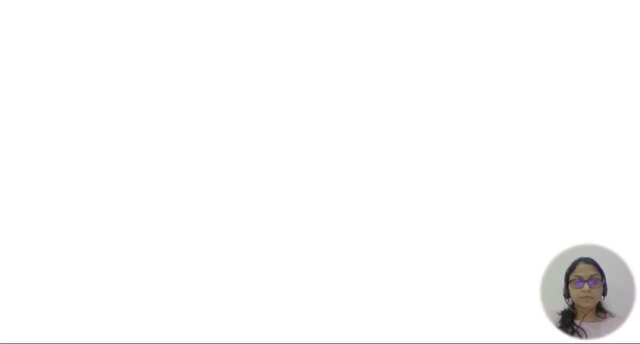 paper and you can touch it, that and you can carry that air to anywhere. so hard copy means um information that is printed on paper, you call it as a hard copy if the same information, if you are able to see on the monitor, means that you call it as a soft copy. so the next, uh, most important part. 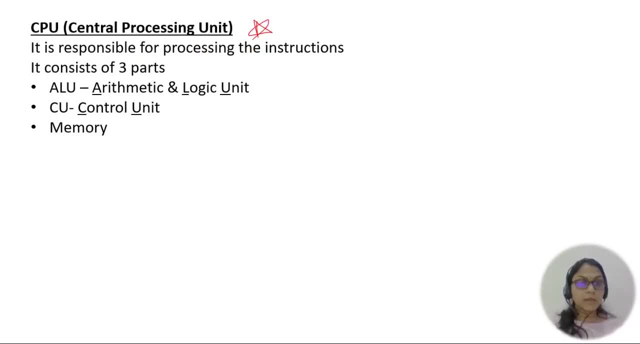 in the hardware component is the cpu. cpu- you call it as a heart of the computer, central processing unit, so you also call it as a processor. then the name of the cpu is the processor, processor which performing the operations, processor performing operation. so it is responsible for processing the 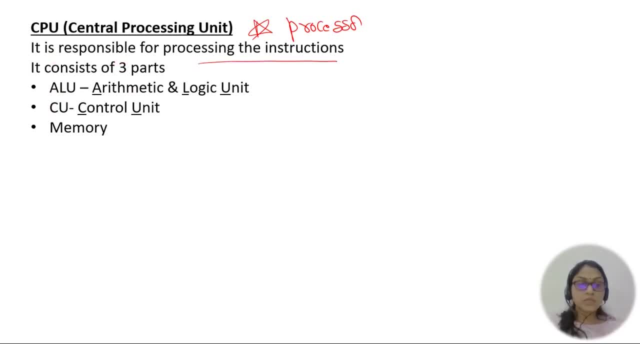 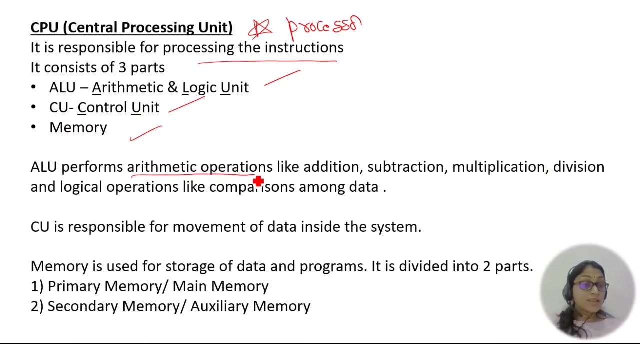 instructions. whatever the instructions that the user has given, those instructions are performing by the cpu. so, generally, the cpu consisting of three parts, one is alu, arithmetic logic unit, cu control unit and the memory. so what is this alu? alu is performing arithmetic operations. arithmetic operations. 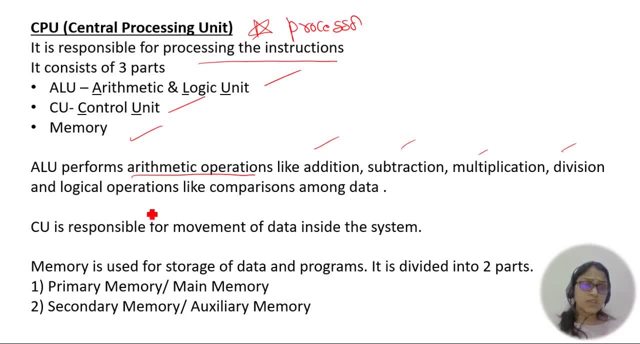 means nothing but addition, subtraction, multiplication, division and logical operation like comparison among the data. everything these are all comes under the arithmetic logical operations. so these arithmetic uh logical operations are performed by one circuit in the post in the processor. alu circuit is there that is going to perform this operation? arithmetic logic unit. 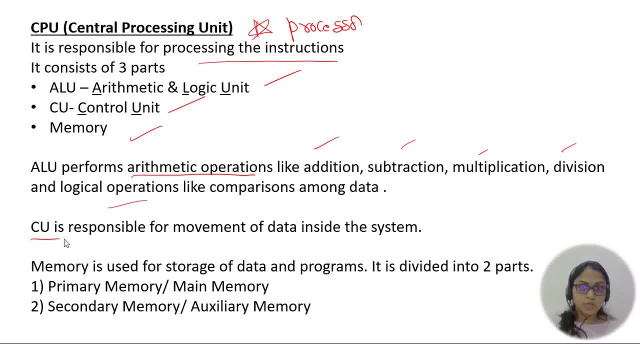 then what about? cu? cu is nothing but the control unit. so what is it doing? it is responsible for movement of data inside the system, if you want. if the data wants to move from one place to enter place, obviously it has to move, because i am the user. i am entering some instructions. 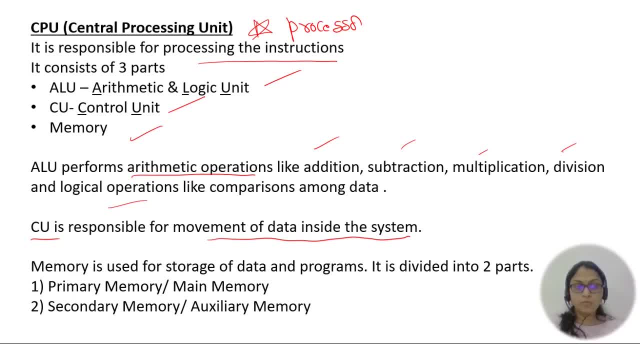 instructions. these instructions has to be passed to the CPU to perform the operation. So this path will be managed by the control unit only. So the control unit is responsible for movement of data from user to the system, to the CPU. So the movement of data inside the system, everything. 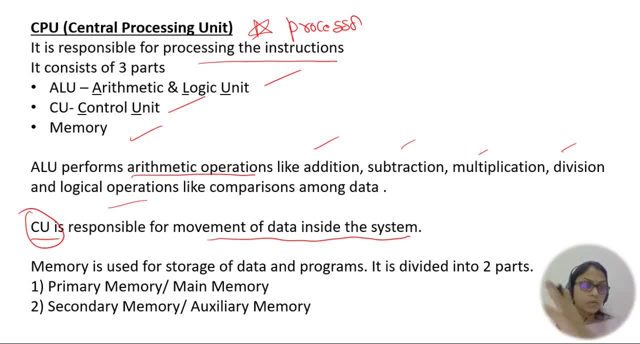 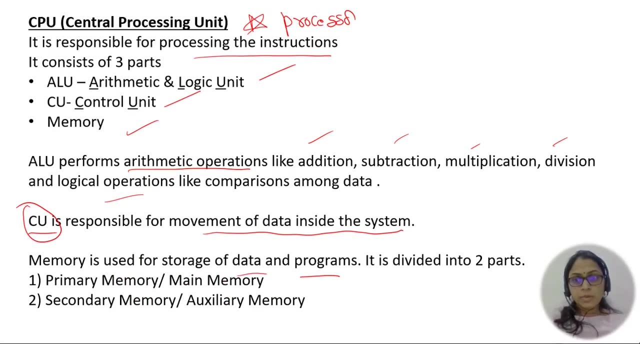 inside the system, the movements of data from hard disk to the processor processor to the RAM, RAM to the output device. everything will be based on the control unit And memory is used for storage of data. Memory is nothing, but it is used for storing. So the memory is divided in, is used for storage of. 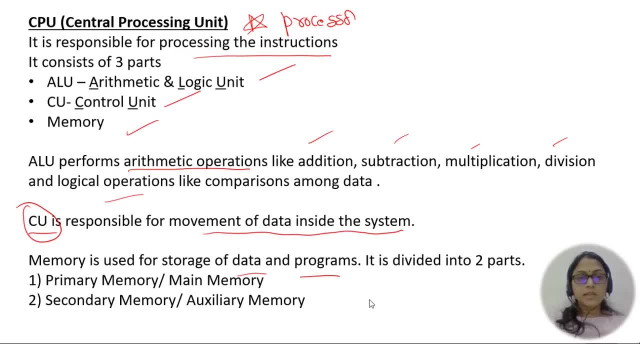 data and program. Okay, and it is divided into two parts. that is what the primary memory and the secondary memory. The primary memory is also called as a main memory. So remember students whenever they used to call as a main memory. So remember students whenever they used to call as a main. 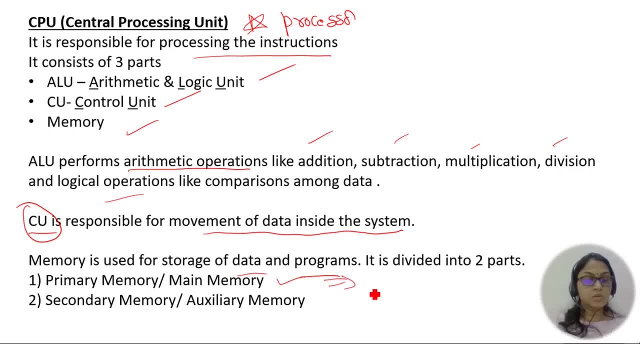 memory. So remember students whenever they used to call as a primary memory. Then the name for primary memory is also called as a main memory, or sometimes we used to call it as a RAM, also random access memory. So these three terms are the same: only primary memory, main memory, random. 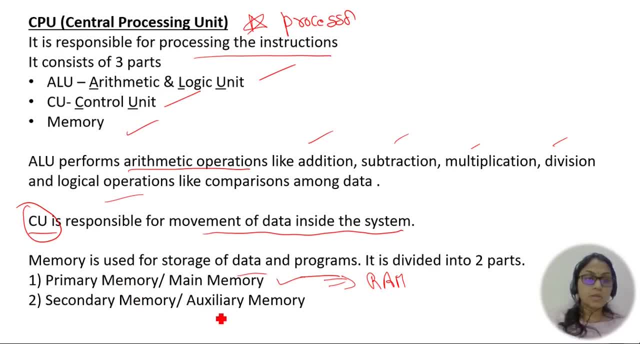 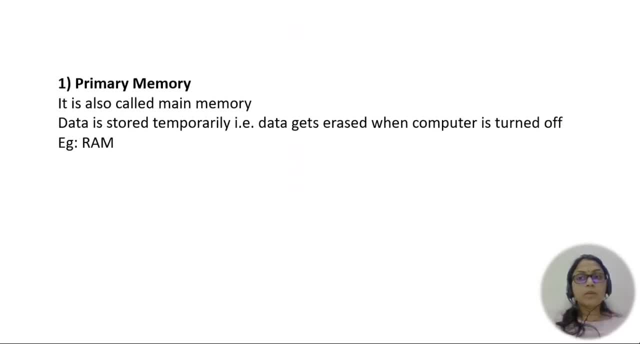 access memory And coming to the secondary memory. the secondary memory is also called as auxiliary memory. Okay, So now coming to the primary memory. So the primary memory. we also call it as a main memory. Here the data is stored temporarily. Here the data is not stored permanently, means it is just stored only temporarily. That is, data gets. 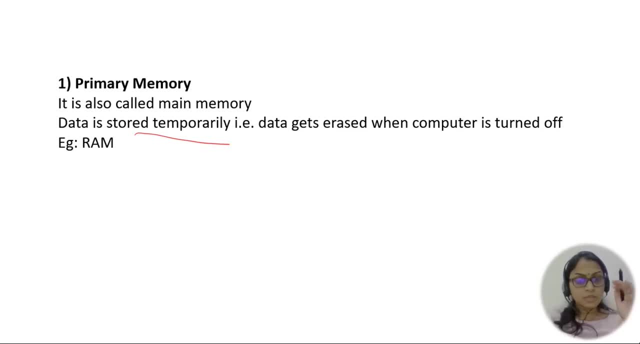 erased when computer is turned off. So whenever your system is on, automatically the complete operating system, the BIOS, basic input output system, everything will be stored on the RAM. And what are the files that you are opened? Okay, Opened those file. complete folders will be stored. 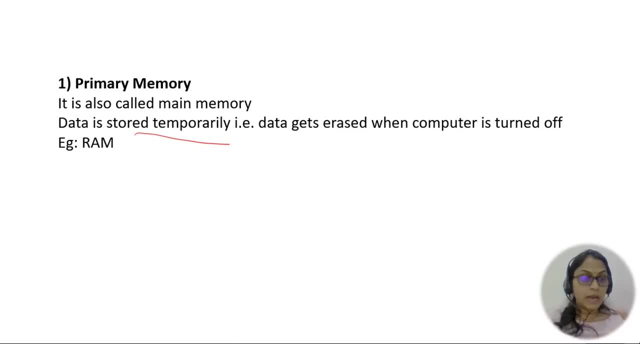 on the RAM. Okay, All the data will be stored until you close the window or you switch off the system. Okay, The data that it is present on the RAM that will be stored until your system is switch off or you have just closed the window. Whenever you close the window, the data here it. 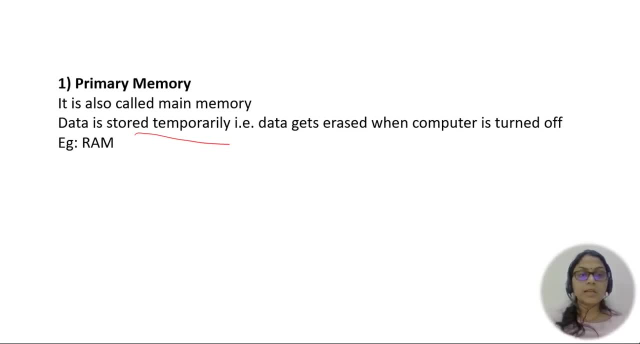 will be lost. Whenever you switch off your system. all the data that is present in the RAM will be erased. Okay, That you call it as a primary memory. Then what about the secondary memory? The secondary memory is also called as auxiliary memory. 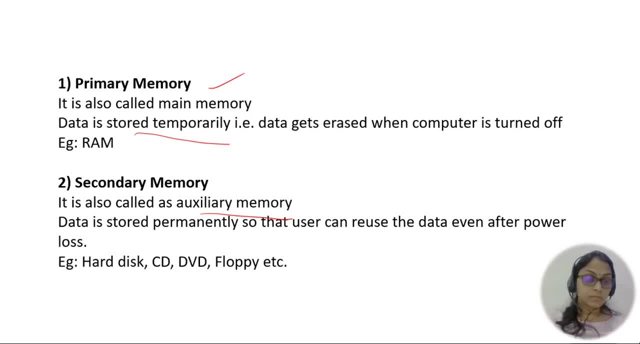 So here the data is stored permanently. Okay, So that user can reuse the data even after power loss. Here the permanently means if you want, you can delete the file. But whenever you switch off your system, the data in the hard disk and the data in the CD, those will not be erased. They. 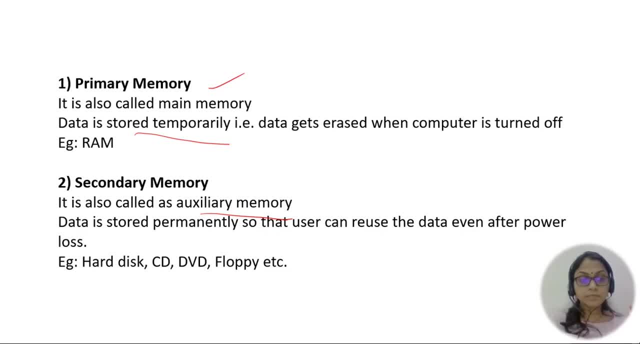 will be stored permanently until you delete. Until you delete. So hard disk means the data is stored permanently. So even though your system is switch off, the data in the hard disk will not be erased. Okay, Until you remove the data And whereas the CD in the CD also, once the data is returned, some 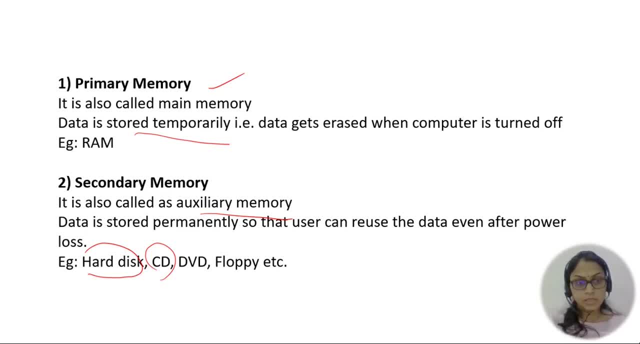 some CDs means it's a rewritable CDs will be there. Readable CDs will be there. So in that also, the data will not be lost. Okay, And coming to the DVD floppies- these are all you call it as a secondary memory. Here the data will not be lost until you delete, Even though your power is switch. 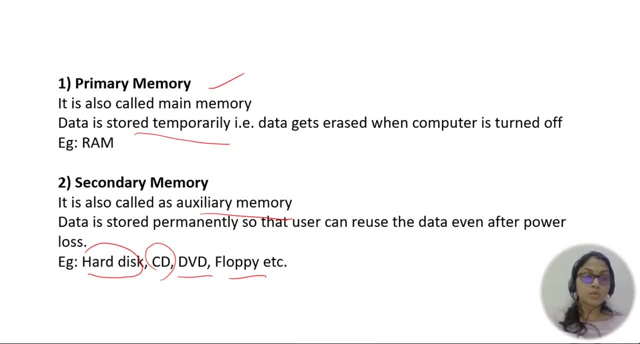 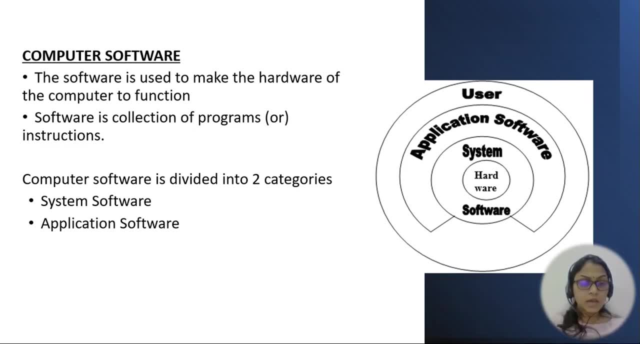 off, the data in those devices will not be lost. That's why we call those are the permanent devices. So that is about the computer hardwares, So what you had seen in the hardware- the input devices and the output devices, CPUs, and the memories You have learned about these things. 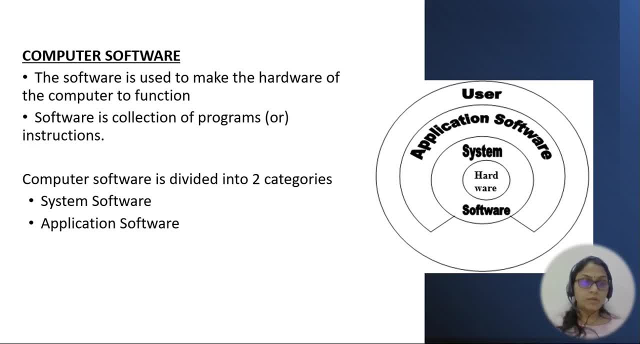 Those are the main components of the computer hardwares, So which you can touch and the feel. Now coming to the computer software, So many people will get a confused regarding what is a computer software and we used to call, like a different softwares, application software system. 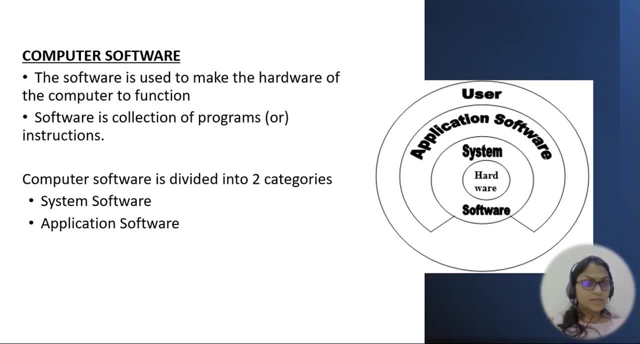 software and what all those things? operating system, what? what about these softwares? So now let's see the difference between all these terms by seeing the concept. A computer software is used to make the hardware of a computer to function If your hardware parts need to perform the operation. 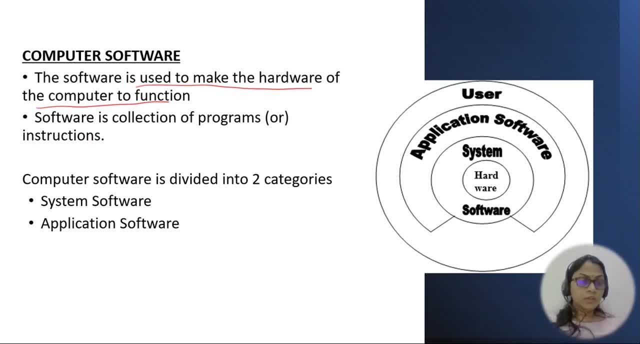 Okay, It has to work. A software should be compulsory. Without software The hardware parts will not perform any operation. So the instructions has to be given with the By using the softwares. A software is a collection of programs or instructions which are given to the hardware parts. So here hardware is there, So the 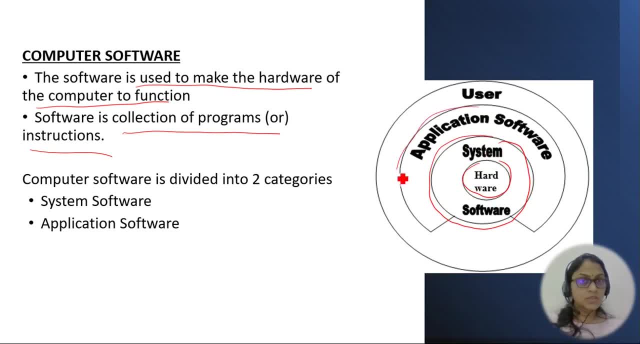 upper layer of the hardware is the system software and next is the application software and the user. user was me And the hardware is a computer Hardware, So interact with the user and the hardware parts. a software should be compulsory, So softwares may. 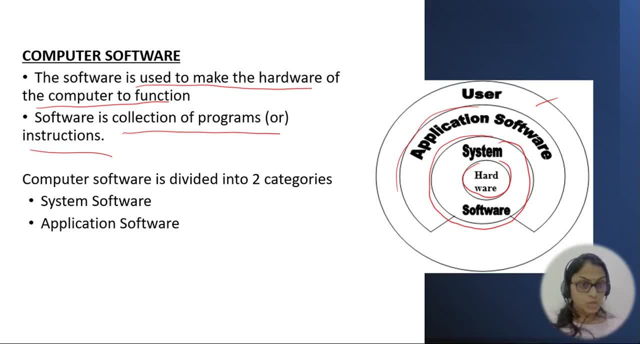 be. the application software should be required and the system software should also required. Both are compulsory, Remember, student. if the user wants to interact with the hardware parts, application software required as well as the system software is also required. A computer software is divided into two categories. One is the system software and another is the application. 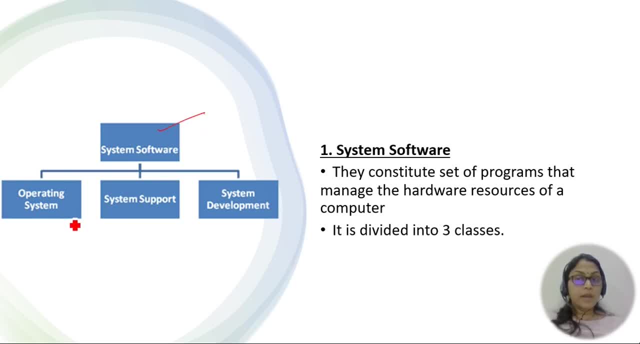 software. Okay again, the system software is generally the system software. you call it as operating system. system support files will be there and system development tools will be there. System software: they constitute set of programs that manage the hardware resource of a computer. 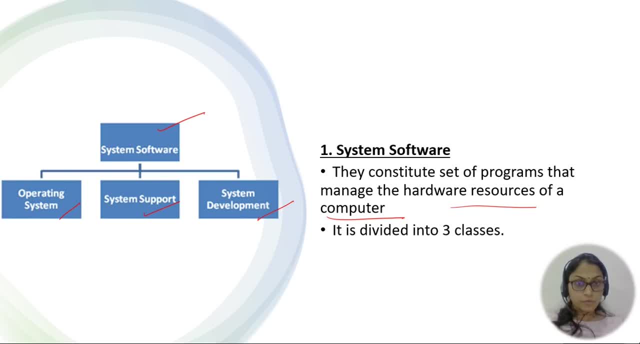 One point you have to remember, student. a system software is used to manage the hardware resource of a computer. It consists of set of programs. Software itself means it consisting of set of programs. Each program is performing some indicating to perform an operation of a particular hardware device. 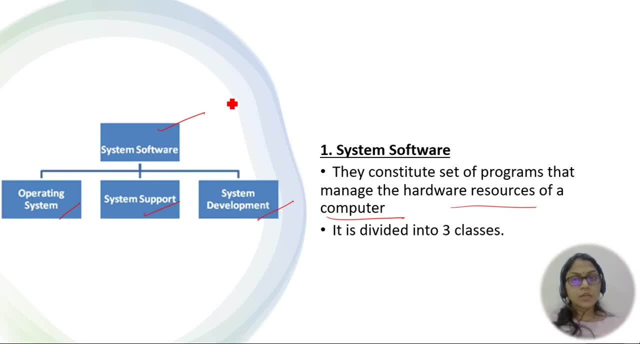 So the system software is also consisting of set of programs, set of programs which are used to manage the hardware resources. So it is going to manage the hardware resources. It is divided into three classes. One is the operating system and there is a system software. So it is going to manage the hardware resources. So it is going to manage the 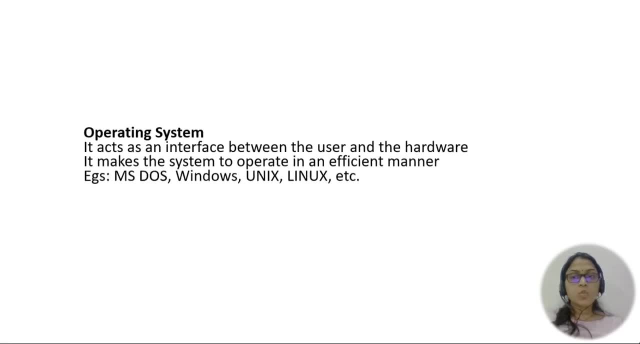 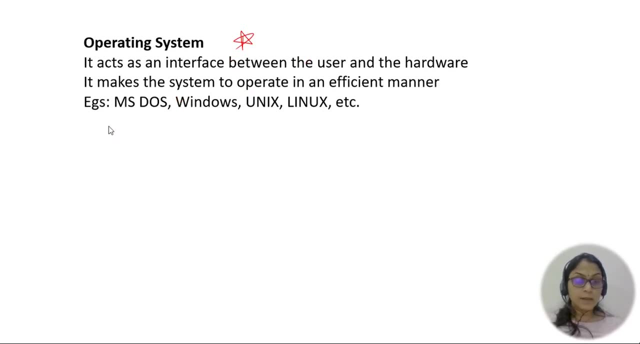 system support. and next is the system development. So what is the operating system, Operating system? you all know about the operating system, right? So if you are working on the laptops means if you are working on desktop means operating system is required. Okay, so different. 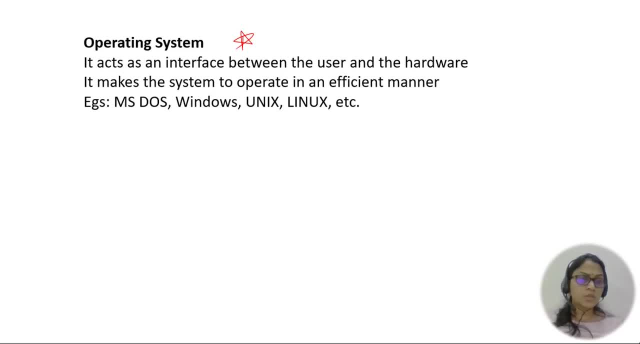 different operating systems are there: Windows, Linux, Unix, MS-DOS. different operating system are there, Based on the user requirements. they can prefer their own operating systems. So operating system acts as an interface between the user and the hardware So to interact with the user has if user wants to interact with the 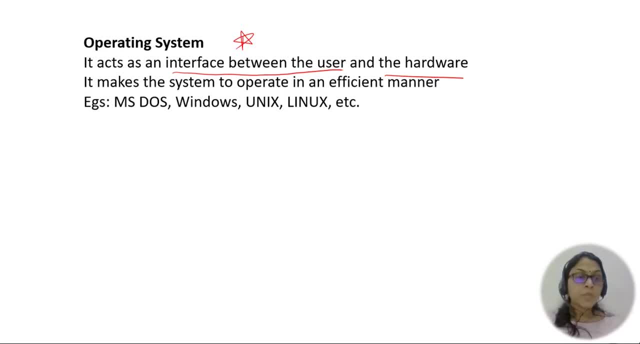 hardware parts means operating system is very important. Without the operating system, no system can perform any operation. So it acts as an interface between the user and the hardware. It takes the system to operate in an efficient manner. Okay, so there are different examples. 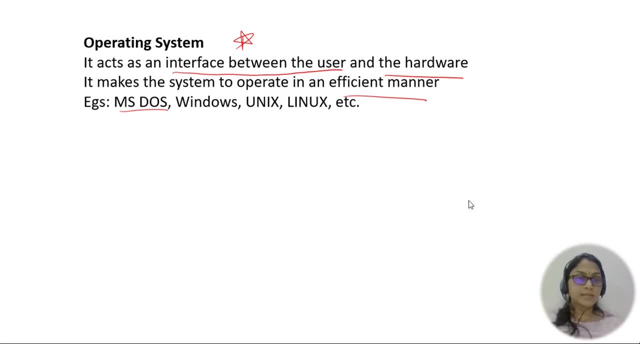 of operating systems or MS-DOS, Windows, Unix, Linux, etc. Now coming to the system support, This system supports provide some utilities and other operating system services. What are those utilities and operating system services? like sort utilities, disk formatting utilities, security. 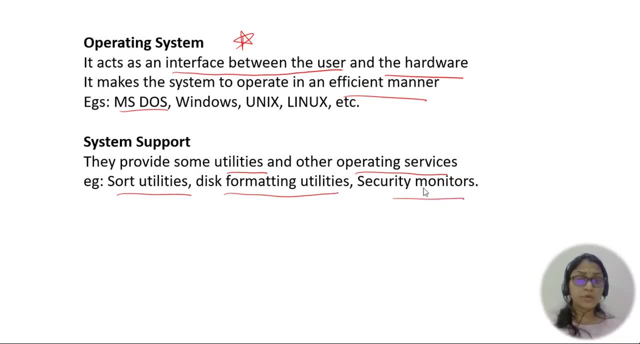 monitor, security monitors. These are all the different utilities that it is going to be provide And system development. So the system development includes language translators, So used for converting programs into machine language. We are the users. We are used to type everything in the high level language, like English, like statements. 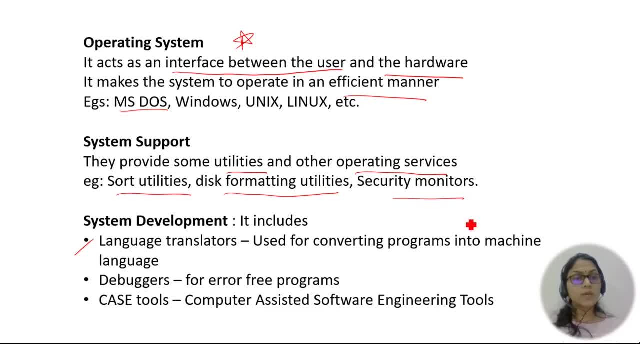 But our system cannot understand the English like statements It's always understands in the form of ones and zeros. Only the machine code it can understand. So the English like statement hi, hello. is going to be converted into machine code. So for this some language translators are: 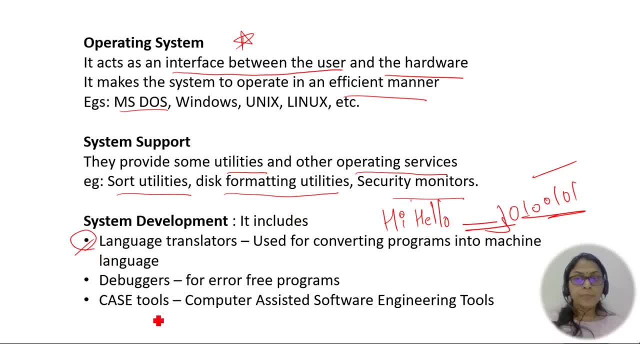 required. So that will be present in the system software And debuggers. Debuggers are used for programs. Some case tools will be present, like computer assisted software. engineering tools will automatic or present in the operating system and the system software, Whenever the user's 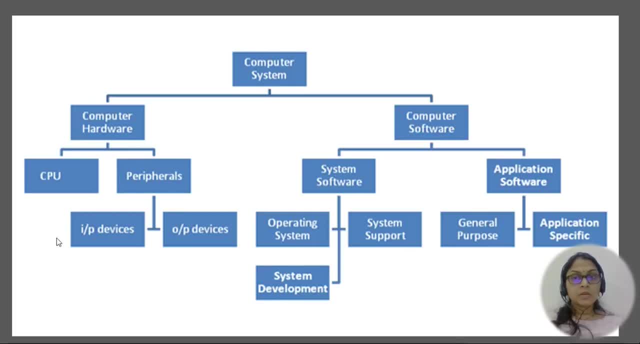 requirement, it can perform the operations. So see here a computer system consisting of computer hardware and computer software. Computer hardware, So the CPU and the peripherals, Peripherals, are nothing but input output devices. Okay, And the memory is also there And computer 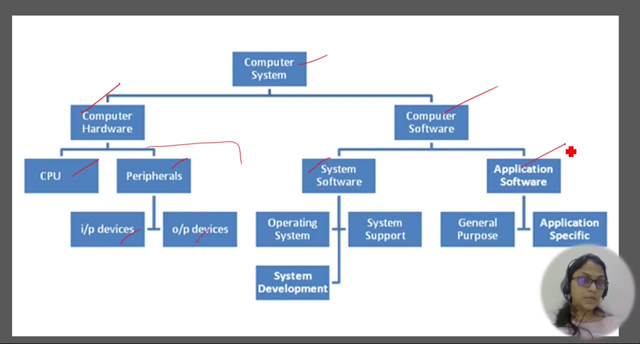 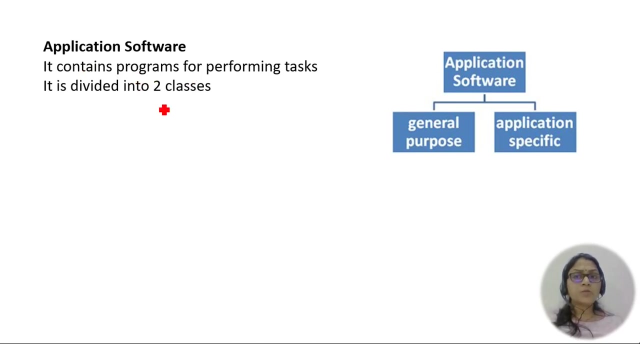 Software. It consisting of system software and application software. System software means just we discussed operating system, system development system. support tools will be there And application software is a general purpose application software and application specific. Let me explain you what is this. application software is So. application software consists of programs for performing tasks. 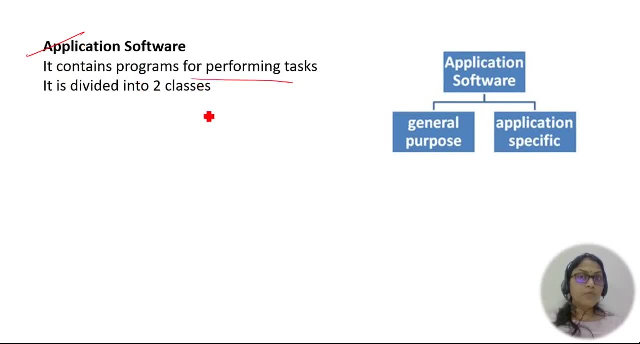 So the main use of application software is it performing tasks? It is divided into two classes: One is general purpose and another is application specific. So what softwares? you call it as a general purpose softwares, General purpose softwares? These are purchased from software developers. If you purchase some softwares from the software developers, 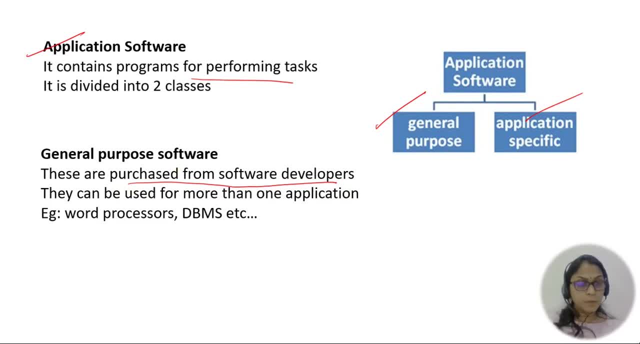 those softwares you call it as a general purpose software. These are not present inside the system software. It will not present inside the operating system. You need to purchase that software to perform the operations. So, based on the user requirements, they can purchase from different software developers. They can be used to for more than one application.